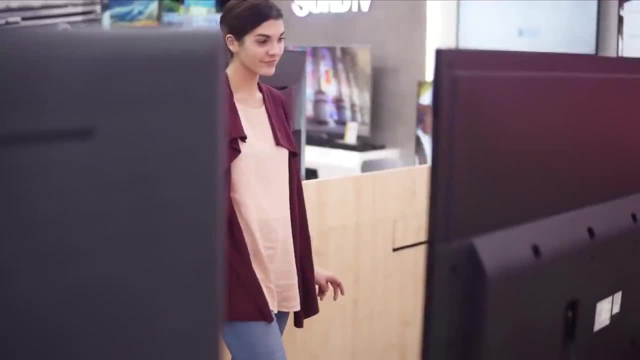 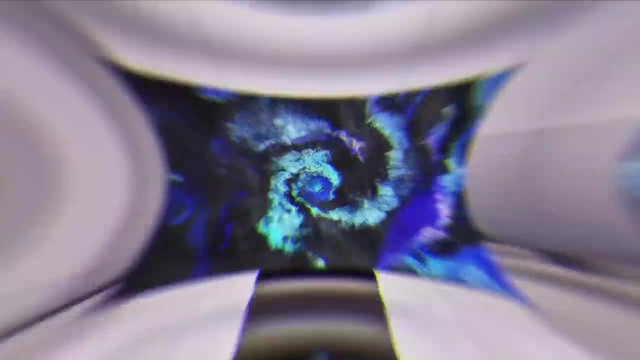 While finding the best TV on the market is difficult because everyone has different needs, you can easily narrow down your search by looking for the best option based on how you're going to use the TV. Each TV has strengths and weaknesses, and there's no perfect TV. 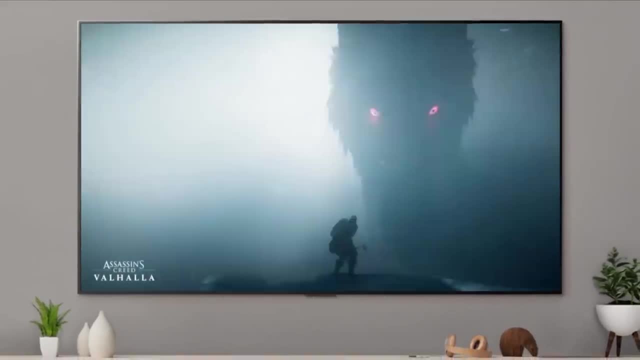 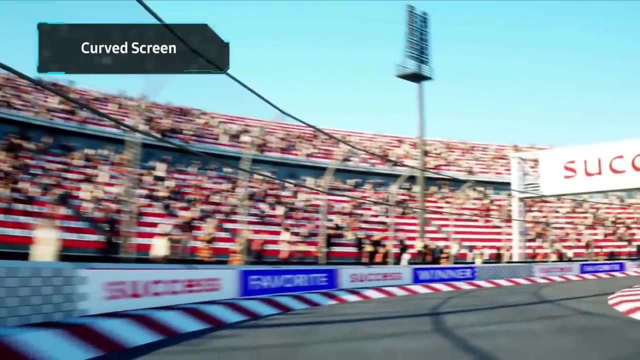 but even the lowest-end 4K TVs offer decent picture quality. The higher-end models are good if you're going to use them to their full ability, like watching 4K HDR content or playing video games. Choosing the best TV on the market depends on how the content you watch. 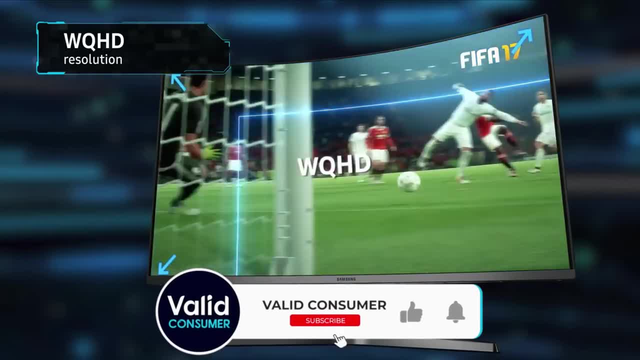 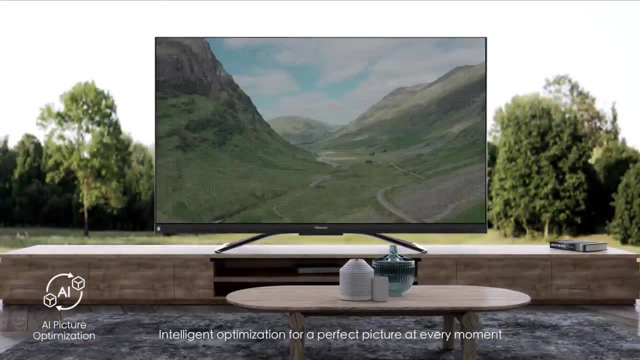 and where you're going to place it. I put together a list of the five best smart TVs that not only address these factors, but also provide great value for your money, And then, depending on your particular situation, you can see which one might be the best option for you. 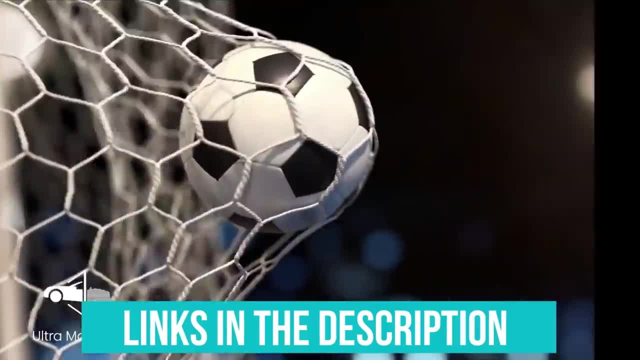 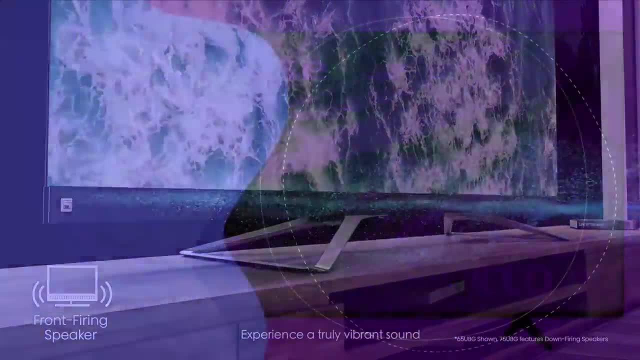 And, as always, you can check pricing for any of these products in the description below And if I'm able to get any discounts or coupon codes, I'll include those for you as well. Now let's get started. Number 5. Hisense U6G. 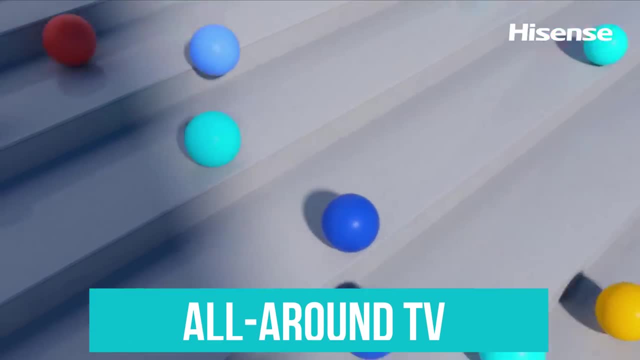 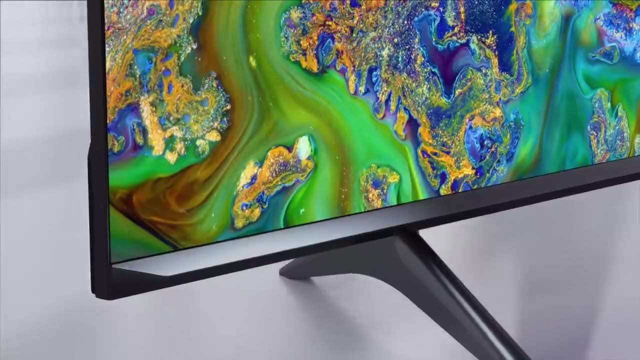 The best budget TV we've tested is the Hisense U6G. It's a great all-around TV that delivers good picture quality and offers performance that rivals some more expensive options. But you won't get some of the same features. For example, it has fewer gaming features than both. 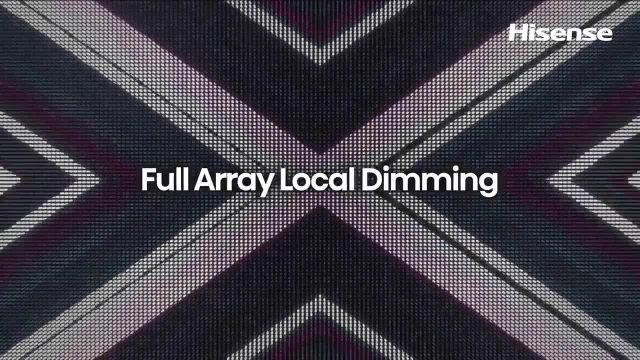 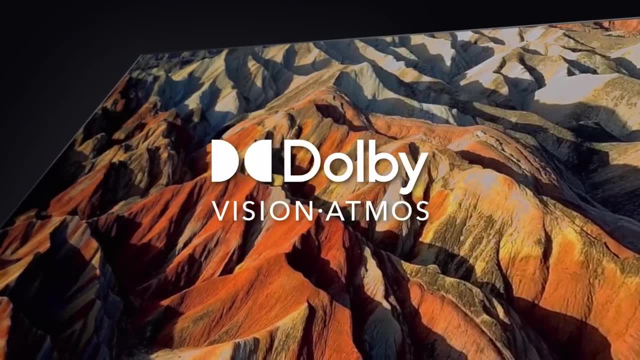 the Hisense U8G and LG C1 OLED, But if you don't need those features, it's a great choice. that'll save you some cash. If you tend to stream a lot of content, you won't have to worry about getting an external streaming device because the built-in Android TV has a ton of 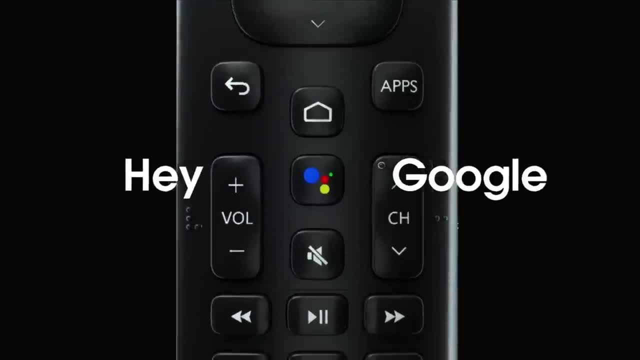 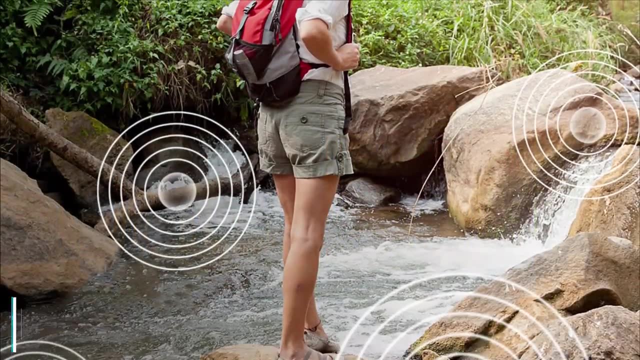 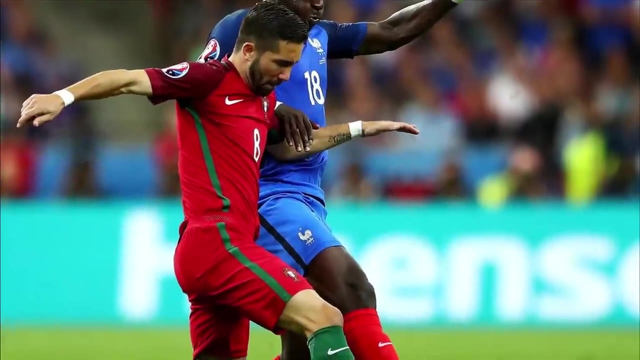 apps available to download, Even if you watch content from a cable box. the picture quality is good because it upscales lower-resolution content without any issue. It's also impressive when watching movies in dark rooms because it displays deep blacks with outstanding black uniformity. Unfortunately, if you want to enhance your movie-watching experience and 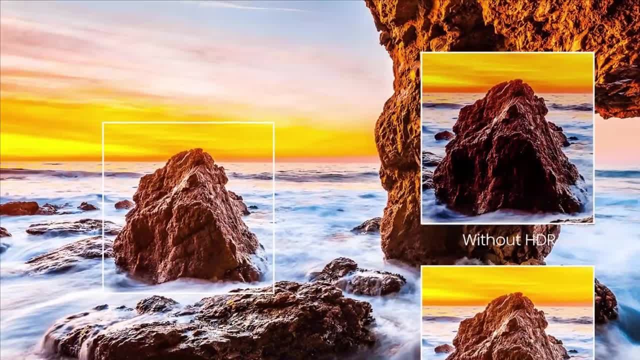 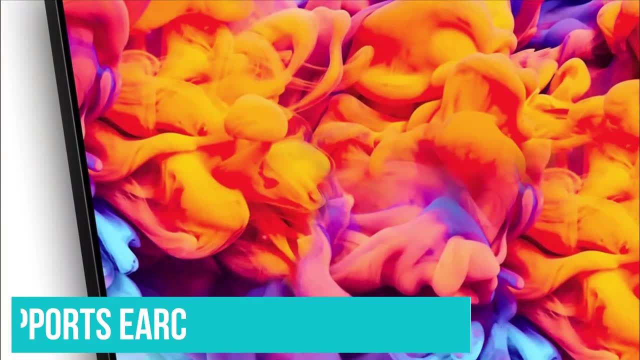 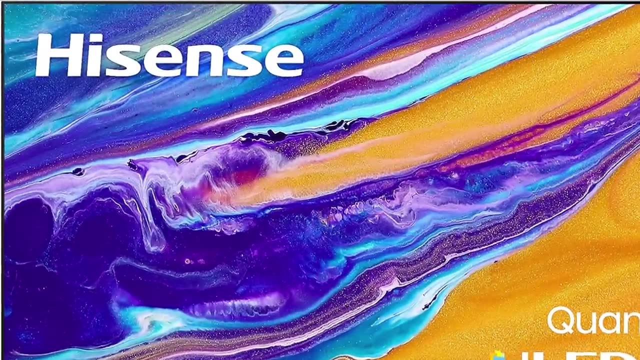 connect a receiver that uses 6G. it doesn't have EARC support to pass high-quality audio formats. If that's important to you, the Hisense U6G-R is similar in performance and supports EARC. However, the U6G delivers the best picture quality for a budget TV and is easier to find. 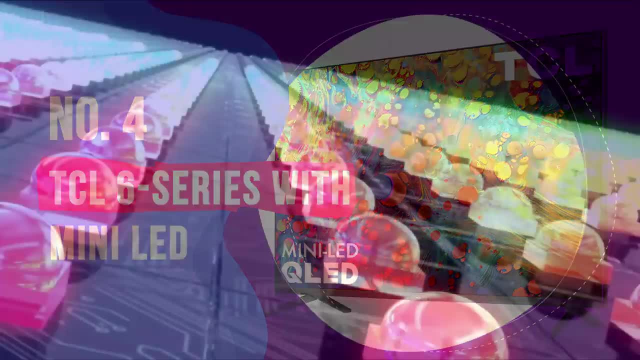 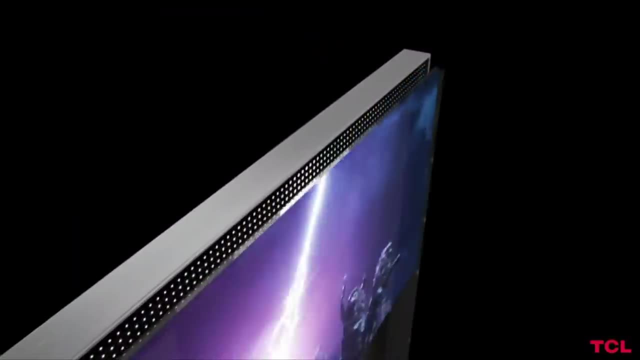 Number 4. TCL 6-Series with Mini-LED. When we discovered that the TCL 6-Series QLED would use mini-LED, we were shocked. That's because just a year prior that same technology came to the high-end 8-Series and cost hundreds. 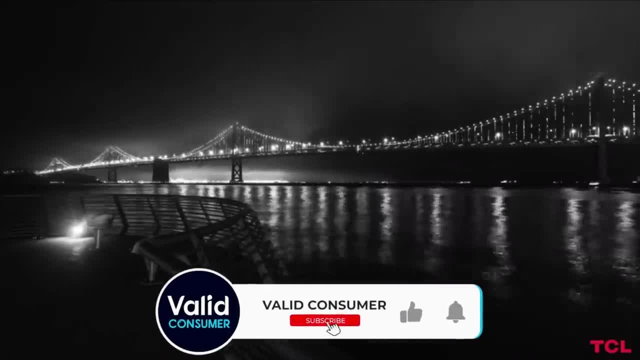 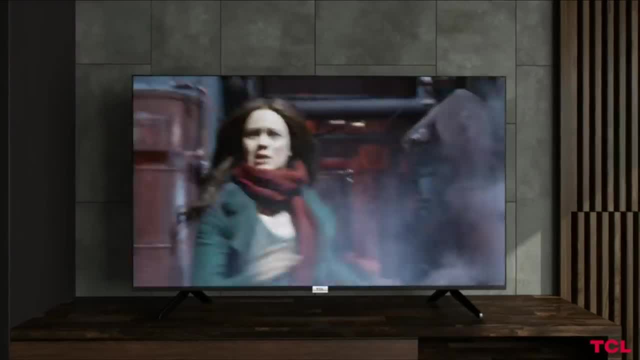 of dollars more than the old TCL 6-Series QLED series. However, the TCL 6-Series QLED series comes with an ultra-affordable 6-Series. It's not the end-all, the all-LED LCD we were dreaming it would be due to its limited brightness and poor motion handling, But it truly is an exceptional. 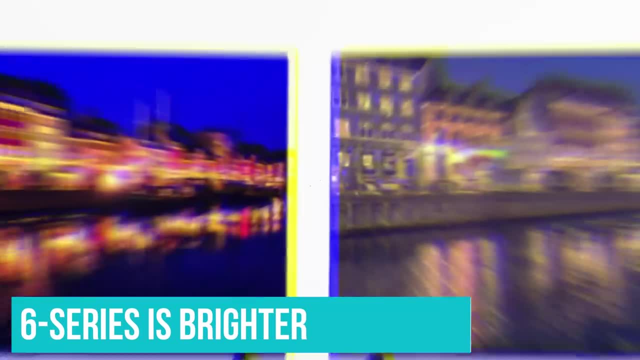 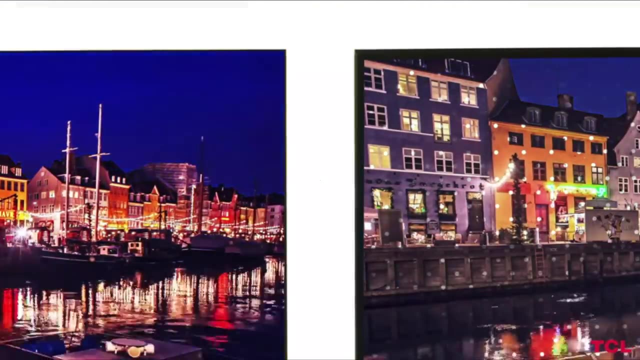 value, and one that we'd recommend to nearly everyone. The 6-Series is brighter than before, more colorful and doesn't have a single hint of haloing or light bleed. It's designed in a new way to hide your cables, and it's the first TV to come. 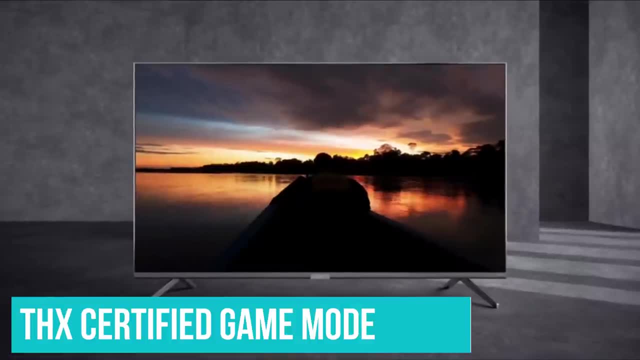 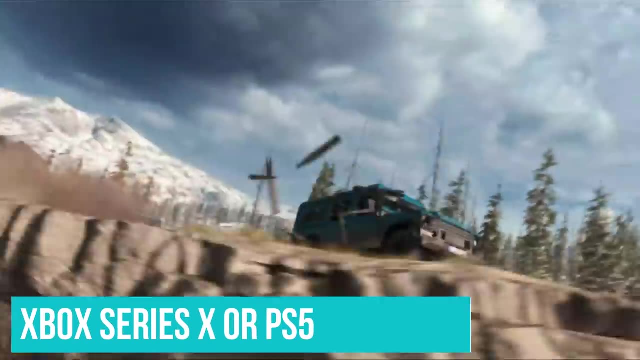 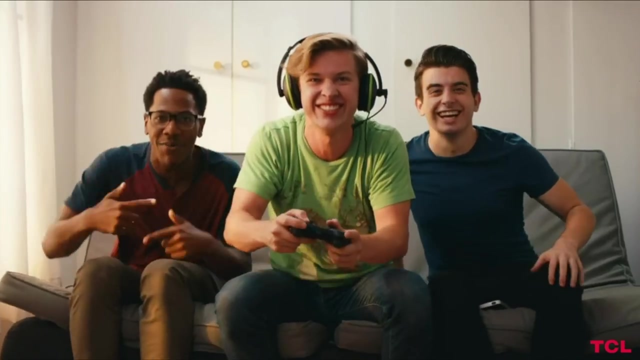 with THX-certified game mode for 1440p by 120Hz gaming. It's not exactly the flat-screen TV we'd recommend to next-gen-ready gamers looking for a perfect companion for the Xbox Series X or PS5 that can push 4K at 120fps. But if you're buying a TV to binge, Netflix, stream Hulu or well, 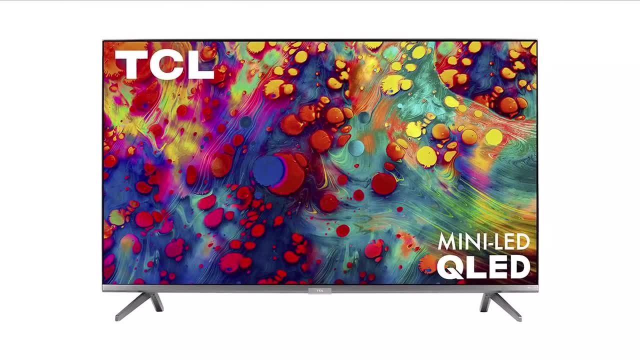 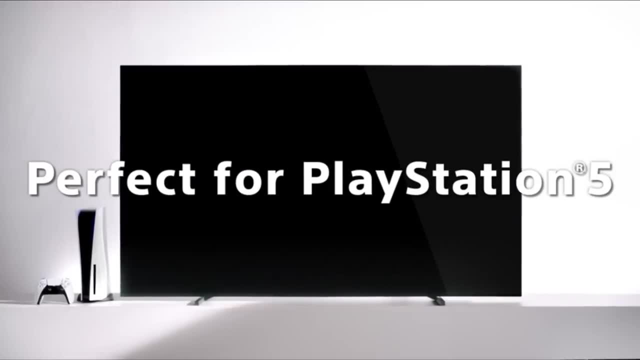 basically just enjoy your viewing experience. this is the best smart TV that we'd recommend for you. Number 3. Sony BRAVIA XRA80J. The Sony BRAVIA XRA80J is one of the best streaming TVs out there, thanks to Google TV streaming and Sony's own BRAVIA Core service. 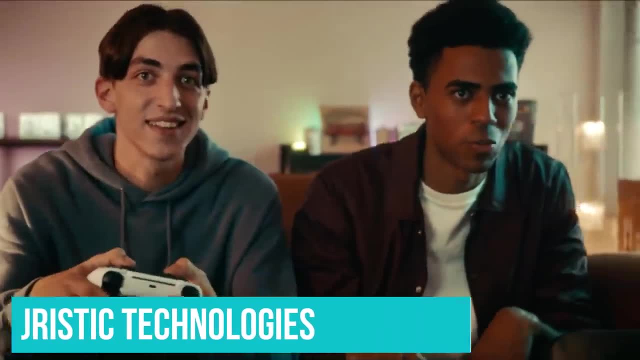 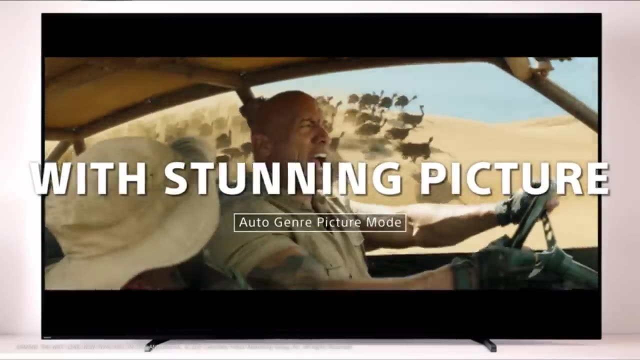 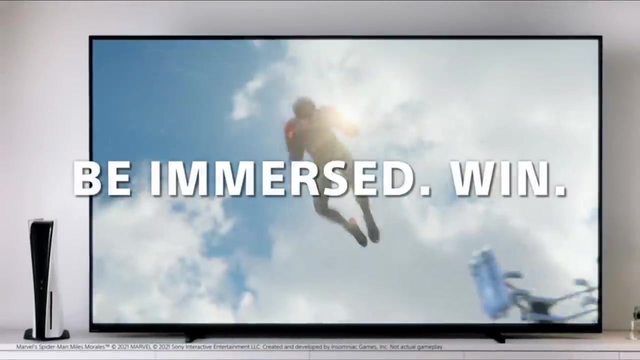 And it's absolutely packed with futuristic technologies. This 4K OLED TV has HDR, a 120Hz refresh rate, ATSC 3.0 tuner, Acoustic Surface, Audio Plus technology. The list goes on. Sure, not everyone will need everything here, but it's nice to have the option. 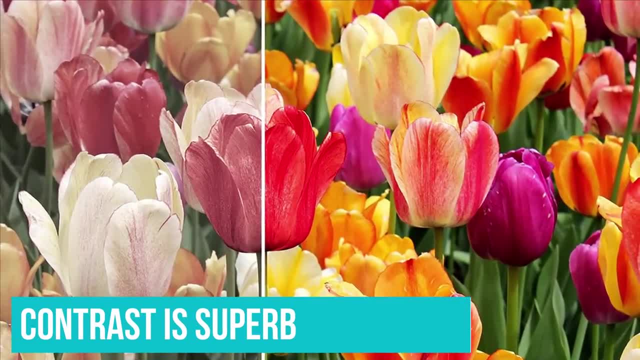 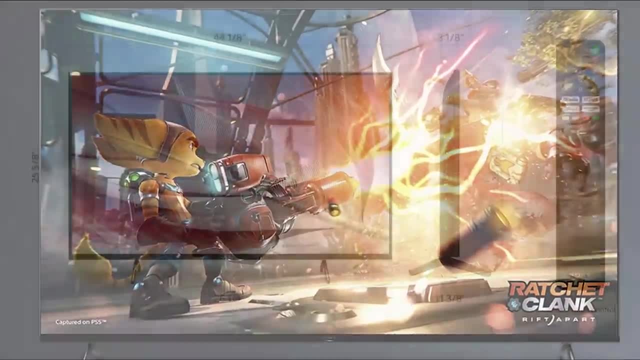 Just as importantly, it also excels at the basics. Contrast is superb, Colors are rich and varied, Viewing angles are impressive and it handles upscaling well. Sound is also excellent and for its smart interface, Google TV is a big upgrade on the older Android TV. 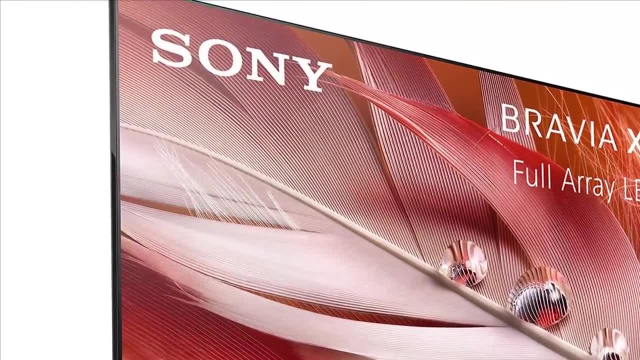 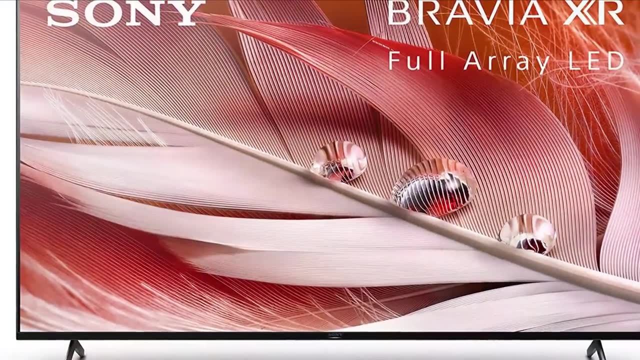 Against that, the XRA80J requires a little more tweaking in order to look its best. It's fine out of the box, but to really reach its full potential you'll want to play around with various modes. It's not the cheapest and other sets beat it. 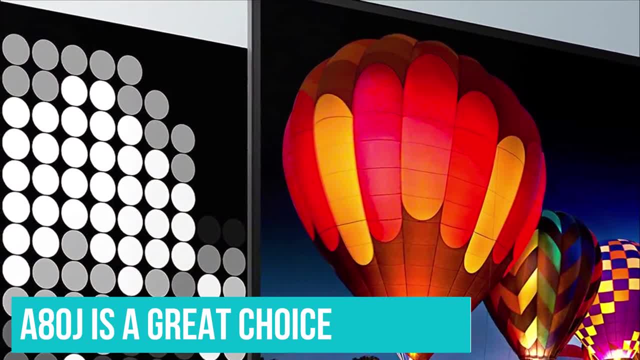 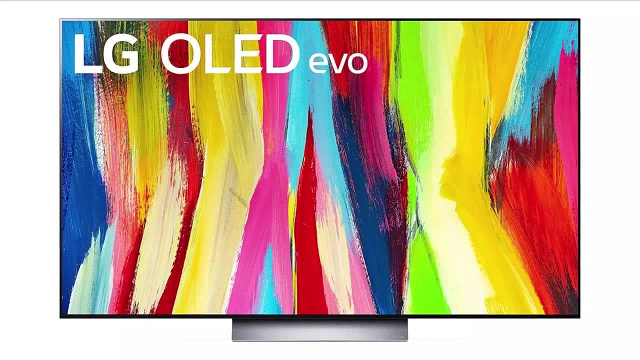 purely based on picture quality, But as an all-round package, the A80J is a great choice. Number 2. LG C2 OLED TV. After dropping a few spots in 2022, the LG C2 OLED reclaims the top spot on our list of the best TVs in 2023.. 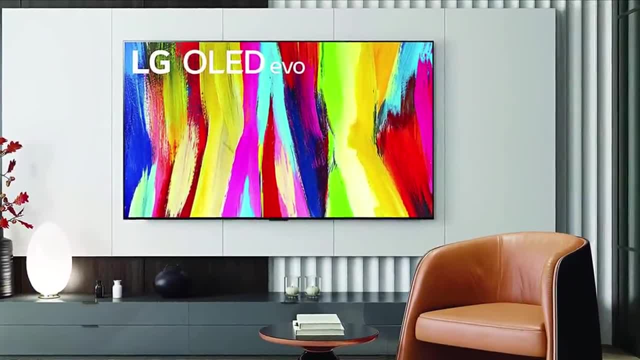 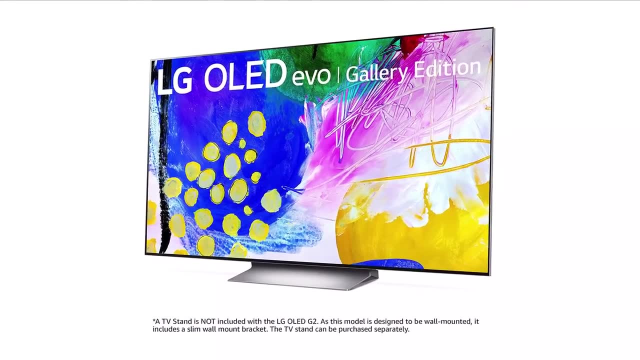 That's due to a number of improvements LG has made to this year's model. compared to the LG C1 OLED. Improvements include the new Alpha A9 Gen 5 processor, which is designed to offer better object enhancement and dynamic tone mapping than its predecessor. As well as that, you're getting 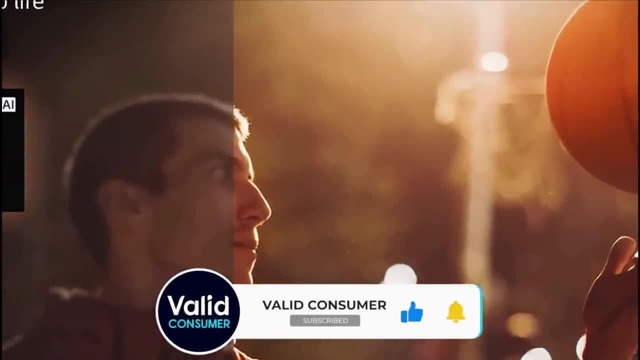 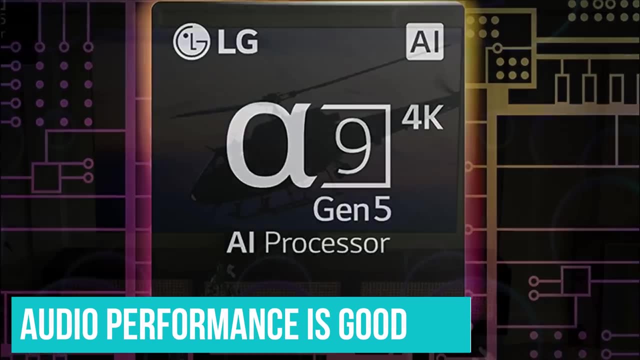 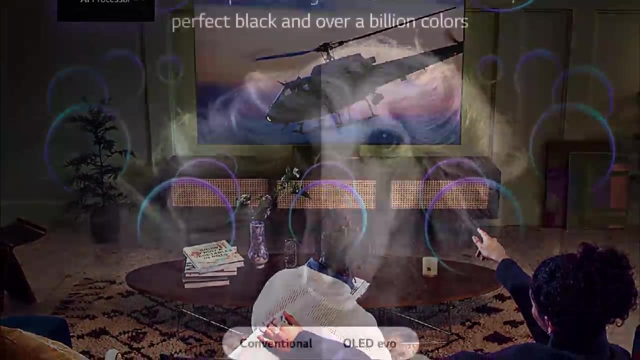 virtual surround sound with the TV upscaling stereo content into 7.1.2 channel sound. While we don't see any changes in the audio performance of the LG C2 OLED TV, we do see some improvements. The audio performance is good for a flat-screen TV and a number of different sound modes means. 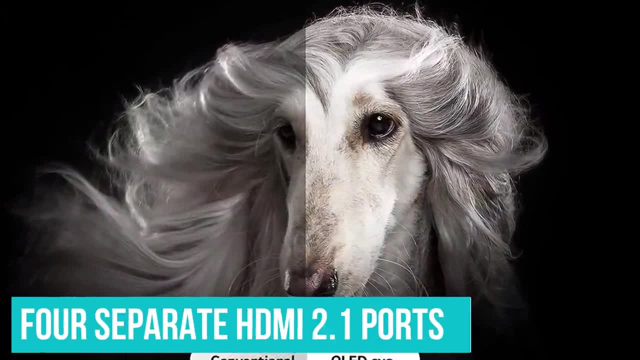 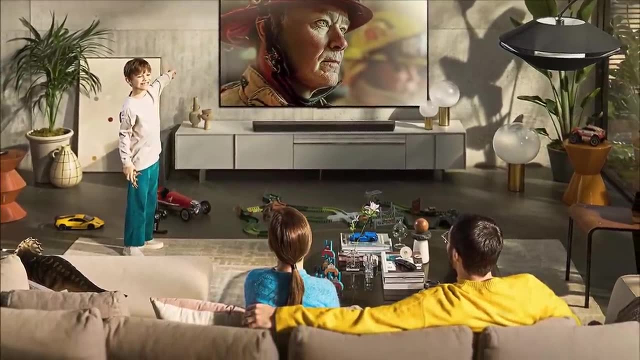 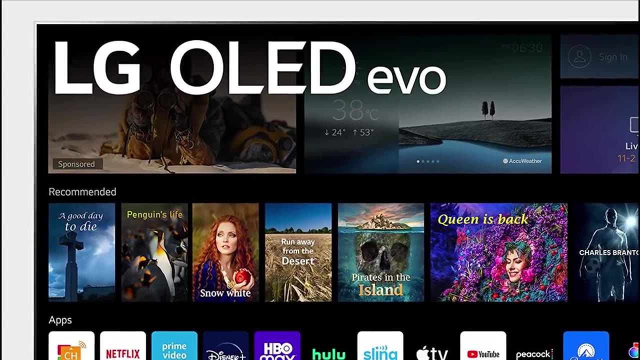 you should be able to find an audio profile that suits your needs. In addition to those improvements, the C2 OLED carries forward the four separate HDMI 2.1 ports that it inherited from the C1 OLED, meaning it's the perfect companion for the PS5, Xbox Series X and Xbox. 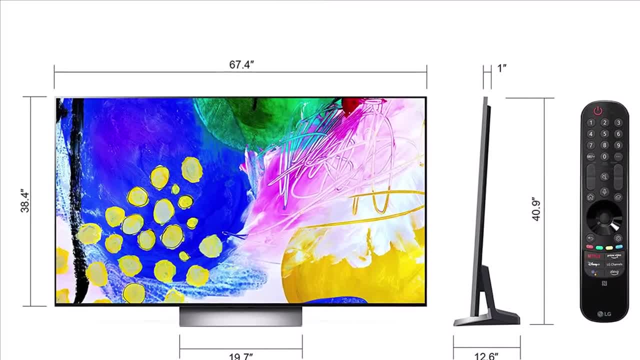 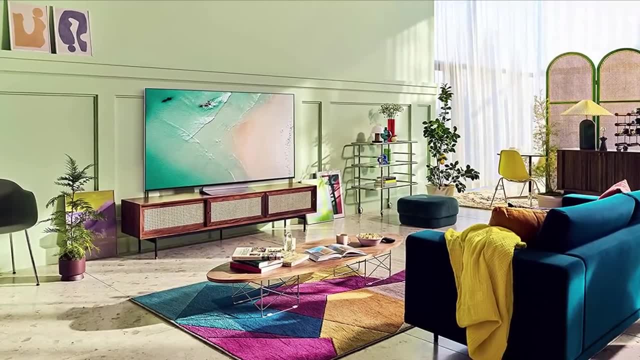 Series S, The LG C2 isn't flawless, however. Off-axis color settings are also great and the saturation does diminish a bit when you move to the left or right of the screen when compared to the new QD OLED models. and LG doesn't support either the IMAX Enhanced or HDR10 Plus format. 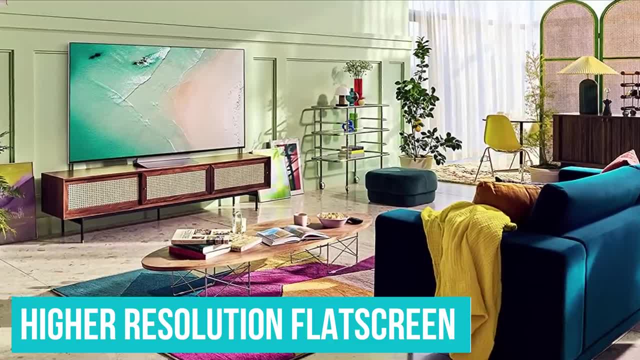 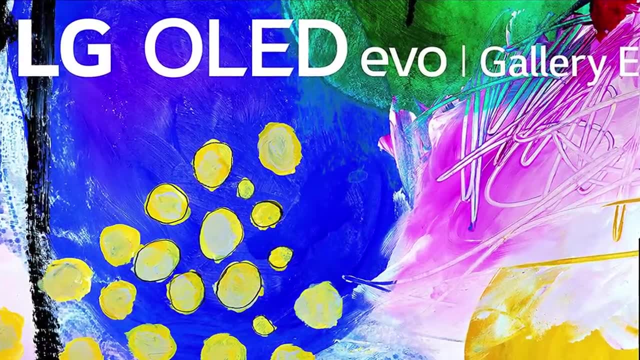 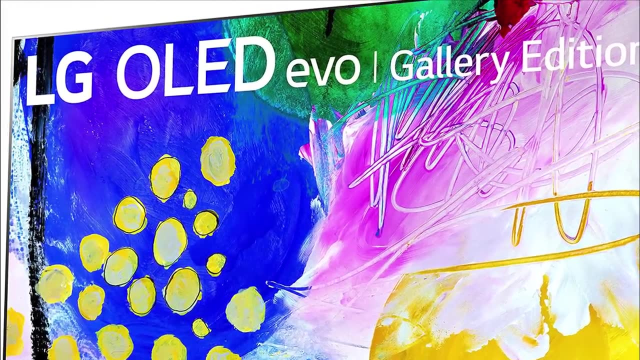 There are, of course, higher-resolution flat-screen TVs out there right now, like the Samsung QN900B, which offers 8K resolution, and the new upgraded LG G2 OLED that has a slightly higher peak brightness, But for the price, this is the absolute best TV you're able to buy in 2023.. 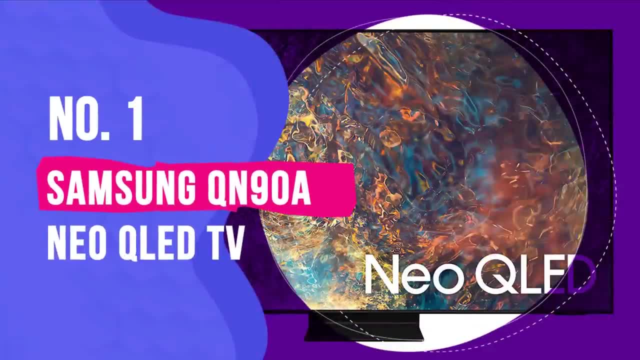 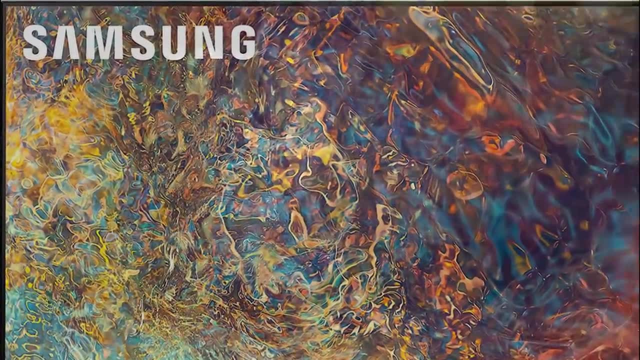 Number 1. Samsung QN90AM Neo QLED TV. The Samsung QN90AM Neo QLED TV combines Samsung's highly refined quantum dot technology with the tight control of mini-LED backlighting, resulting in one of the best TV displays you'll ever see. 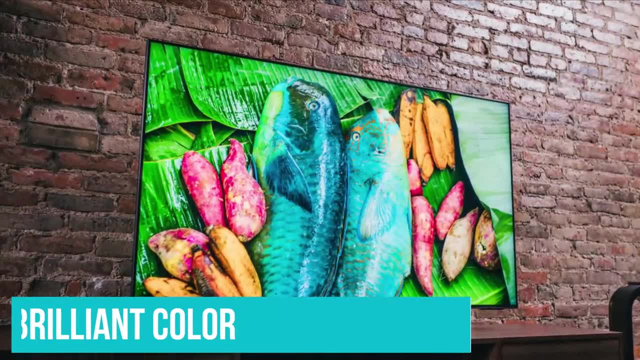 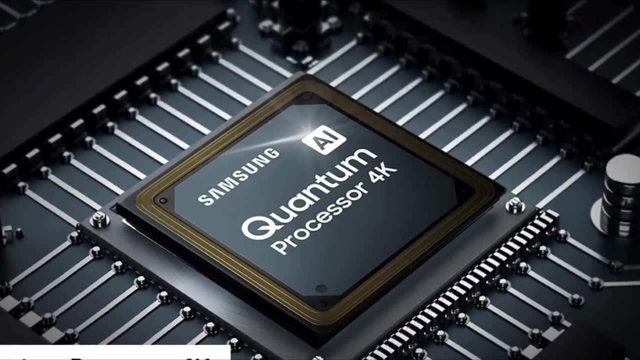 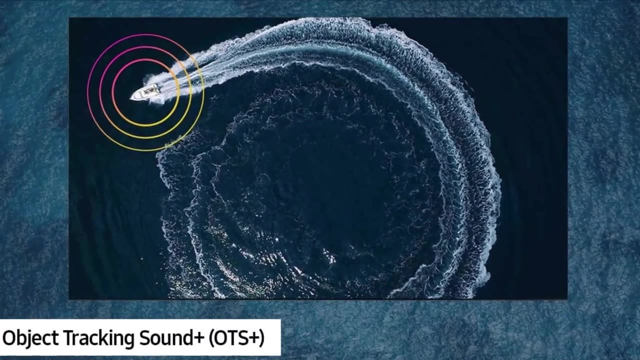 Brilliant color and unmatched brightness make for superb performance, and Samsung pairs that with a bounty of smart TV functions and genuinely intelligent features, like a solar-powered remote control that eliminates the need to swap out batteries, delivering eco-friendly design and unbeaten convenience at the same time.